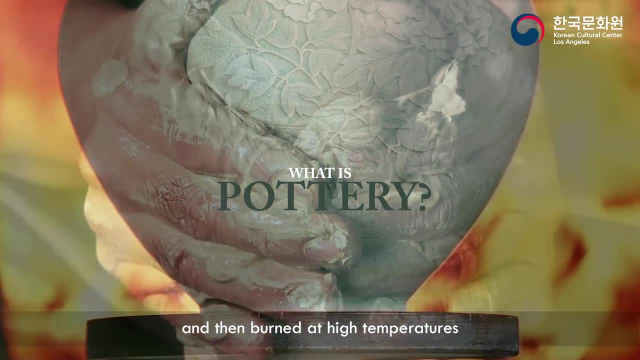 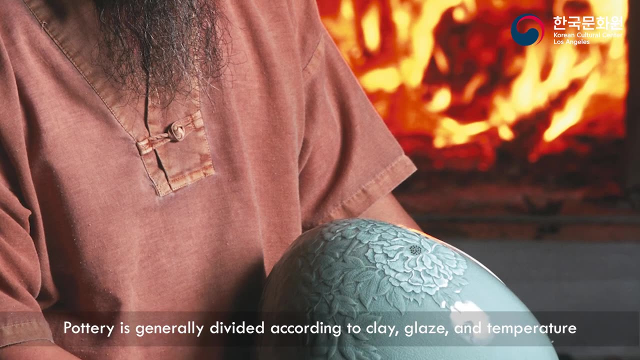 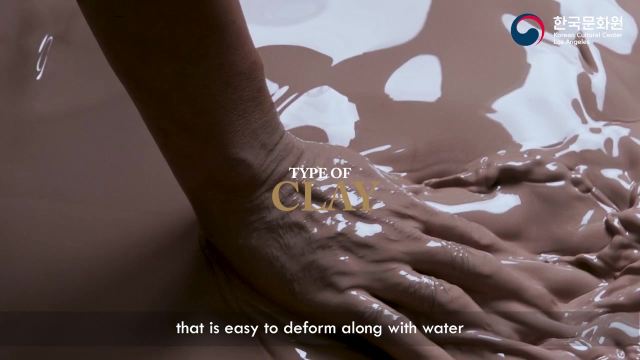 Generally, poro is made of clay and then burned at a high temperature. Poro is generally made of clay and then burned at a high temperature. It is generally divided according to clay glaze and temperature. Poro clay generally uses something that is easy to deform along with water. 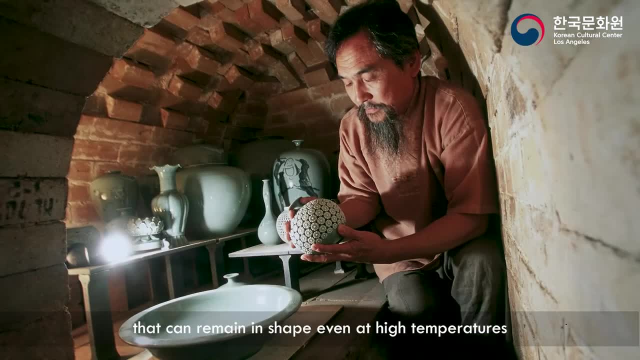 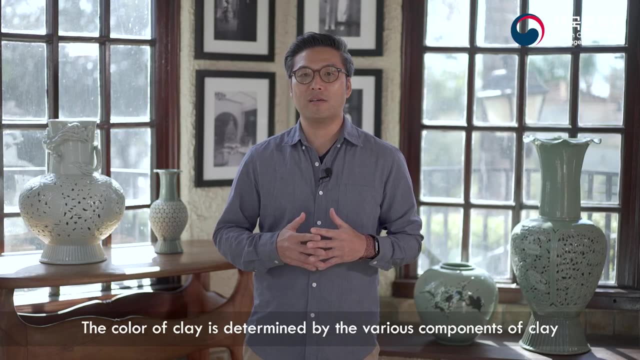 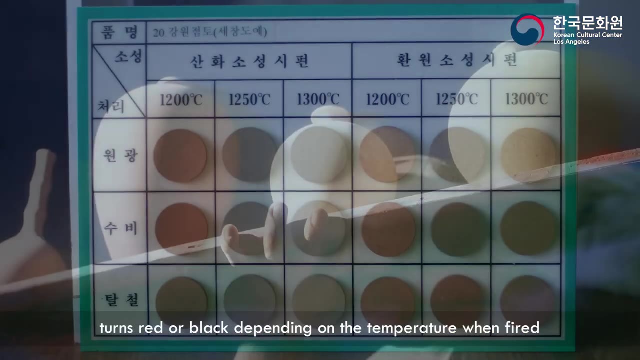 This clay contains a lot of materials that can remain in shape even at a high temperature. The color of clay is determined by the various components of the clay. For example, a clay which has high iron contents turns red or black depends on the temperature when fired. 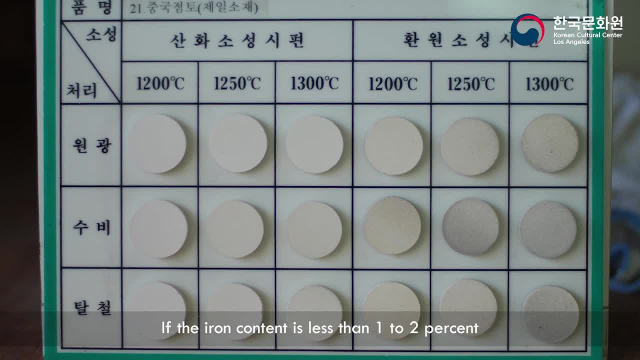 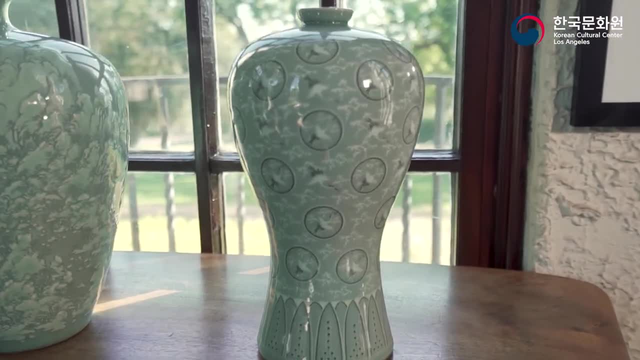 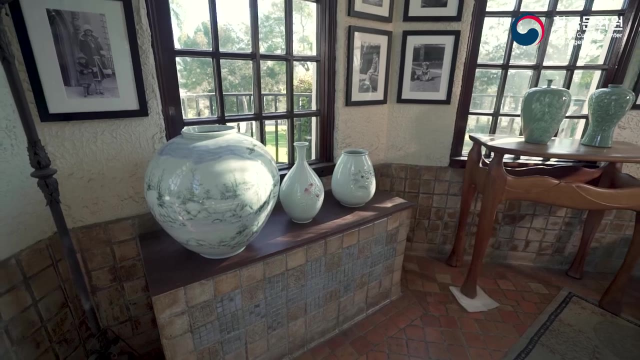 If the iron content is less than one to two percent, it becomes white clay. Please subscribe to my channel if you are interested in learning more about the world of poro. Thank you, Please subscribe to my channel if you are interested in learning more about the world of poro. 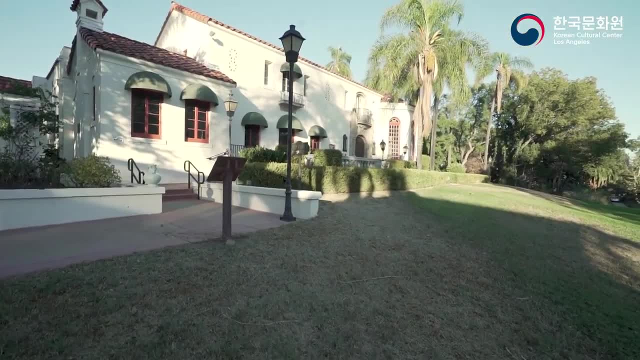 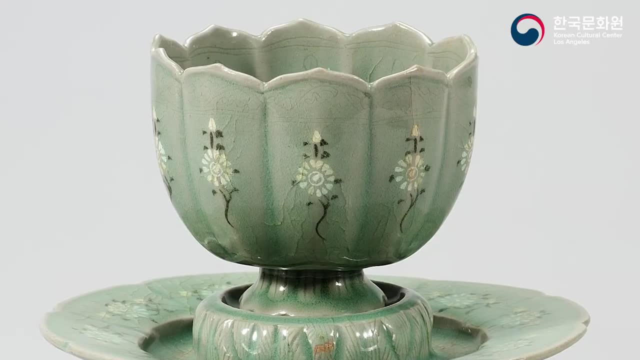 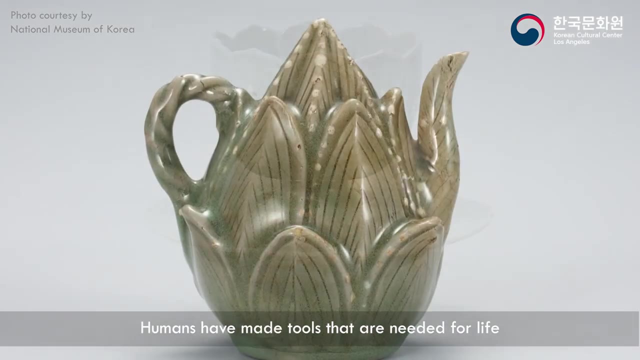 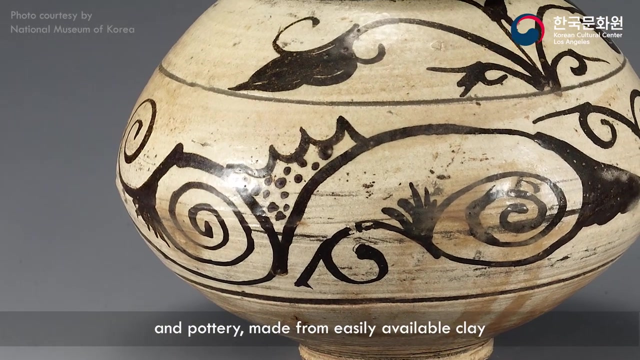 Thank you. The history of pottery began thousands of years ago and is intertwined with the history of mankind. Humans have made tools that are needed for life from materials that are easily available, And pottery made from easily available clay is the origin of today's pottery. 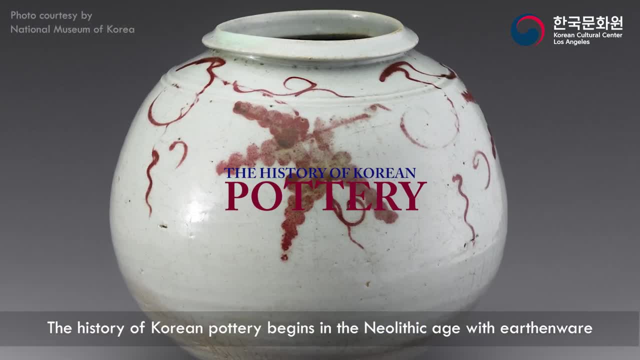 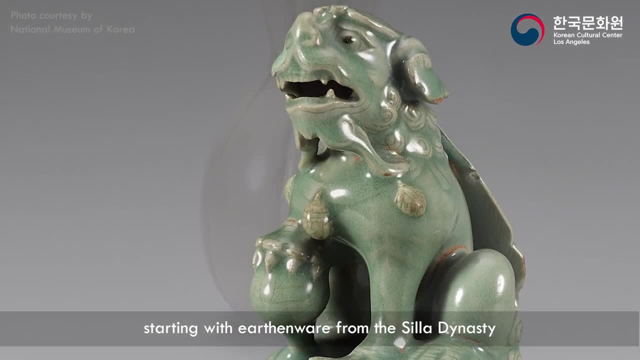 The history of Korean pottery begins in the Neolithic Age with earthenware. As we move closer to our time, Korean pottery production can be divided into different periods, starting from earthenware, from Silla Dynasty, celadon, from the Goryeo Dynasty, punchon, from. 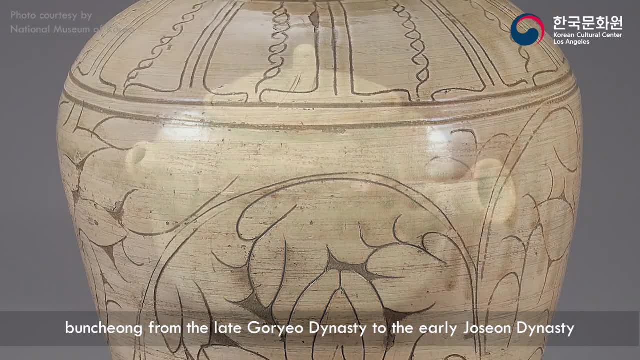 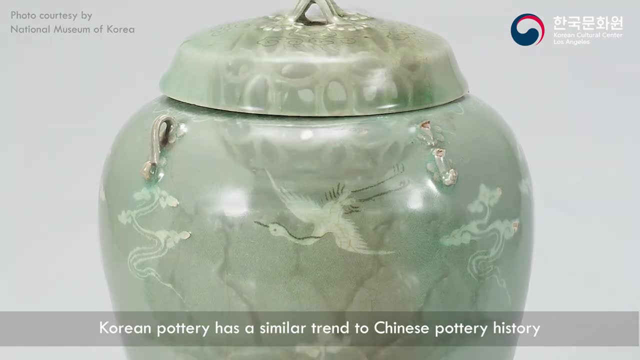 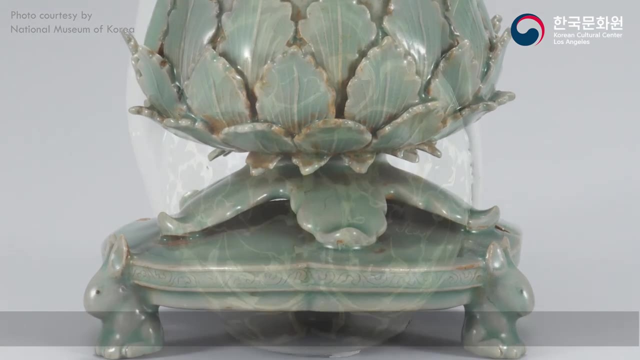 the late Goryeo Dynasty to the early Joseon Dynasty and white porcelain from the Joseon Dynasty. Korean pottery has a similar trend to Chinese pottery history. However, Korean pottery is slightly different. It is different in design, color and method of production from Chinese pottery. 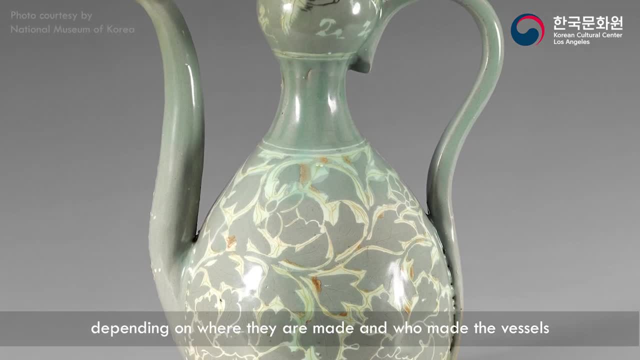 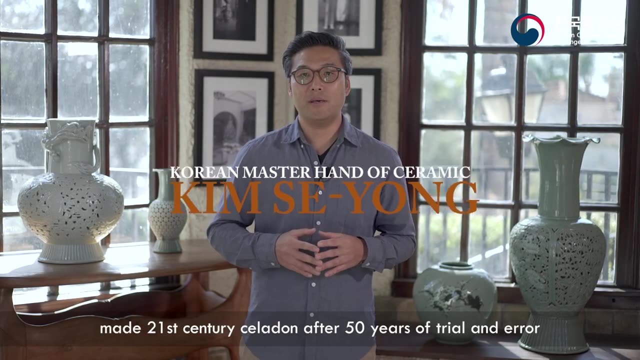 This is because the materials and techniques of pottery vary depending on where they are made and who made the vessels. Kim Se-young, Korean master of ceramics, made 21st-century celadon after 50 years of trial and error to recreate Goryeo Celadon. 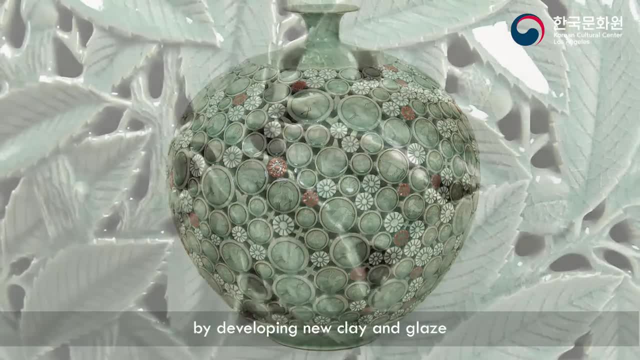 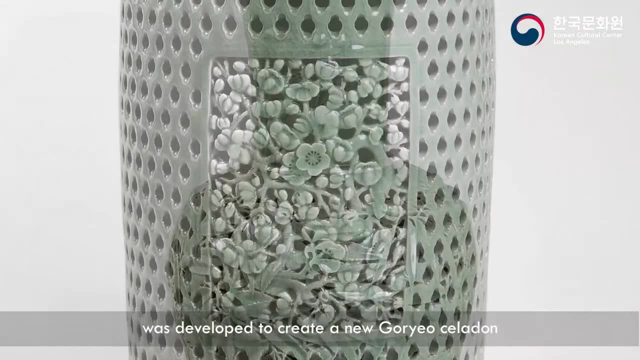 He recreated the beautiful color of Goryeo Celadon by developing new clay and clays. In addition, a double-opening process is required. In addition, a double-opening process is required. In addition, a double-opening process is required. A double-open-work technique was developed to create a new Goryeo Celadon as a groundbreaking. 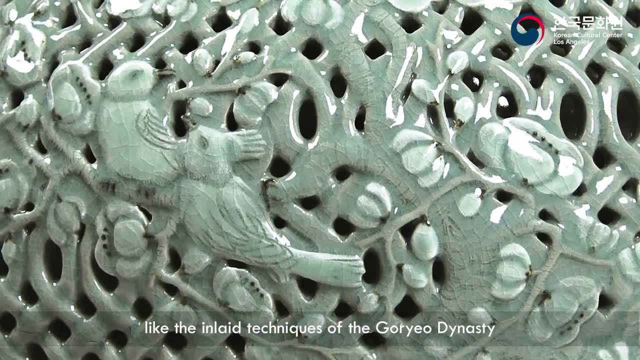 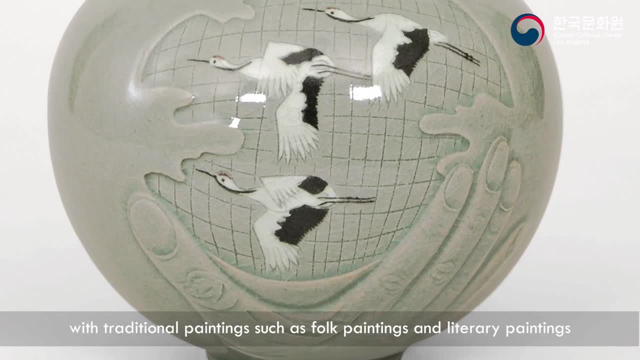 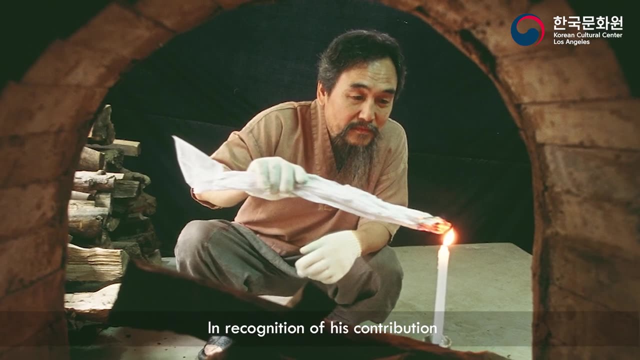 technique, like the inlaid technique of the Goryeo Dynasty. He developed a new style and design by combining the traditional patterns of Goryeo Celadon with traditional paintings such as folk painting and literary painting. In recognition of his contribution, he became a Korean master of ceramics, awarded by the 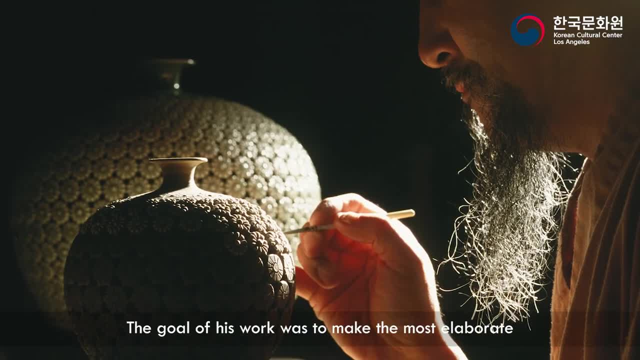 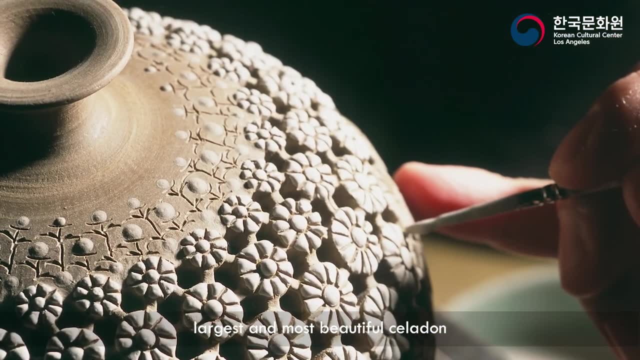 Korean government. In recognition of his contribution, he became a Korean master of ceramics, awarded by the Korean government. In recognition of his contribution, he became a Korean master of ceramics, awarded by the Korean government. His 50-year journey is still ongoing. 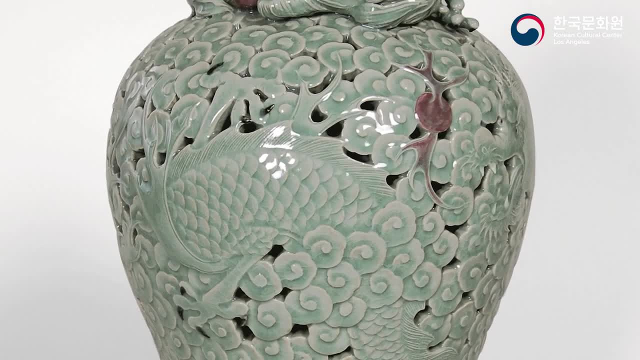 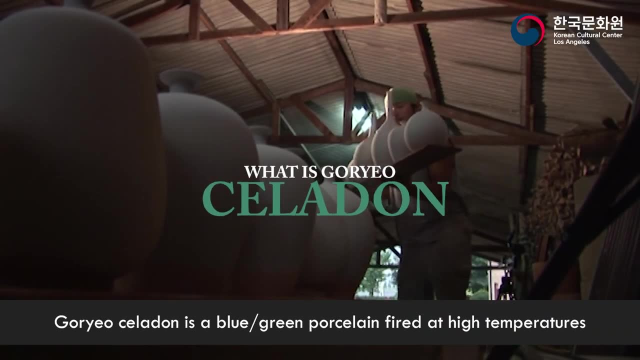 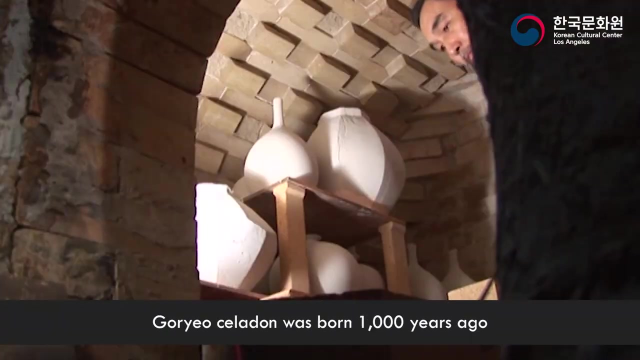 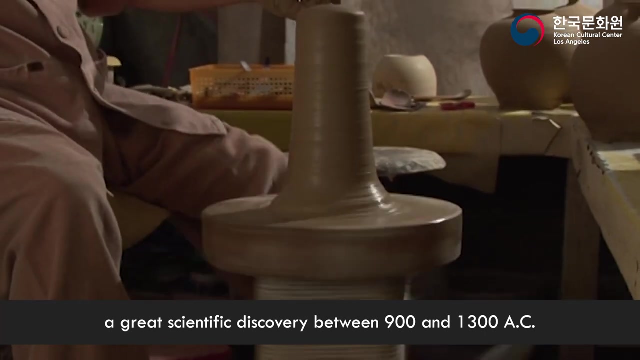 Corioceladon is a blue-green porcelain fired at high temperatures. It was created by Koreans' indomitable will to adapt to poor conditions. Corioceladon was born 1,000 years ago, a great scientific discovery between 900 and 1300. 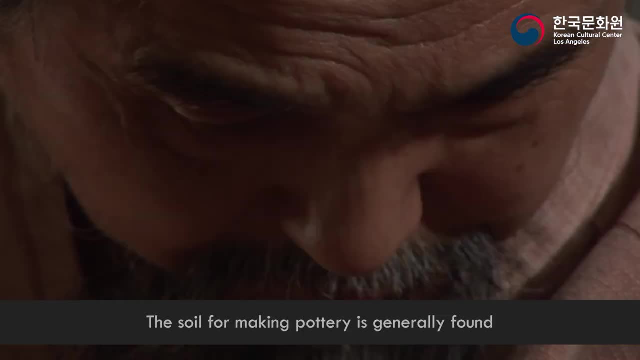 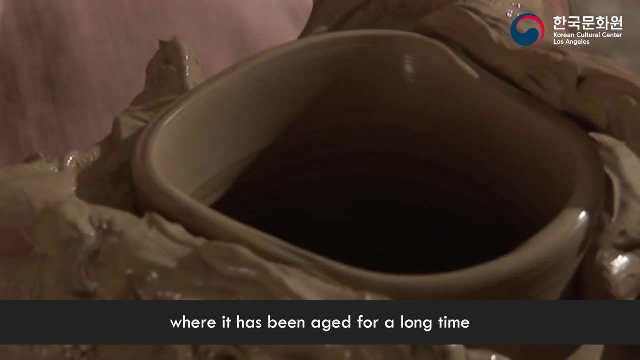 AC, which exceeded the limits of materials. The soil for making pottery is generally found in old areas of the earth's surface where it has been aged for a long time, But the clay of Corioceladon was not made of this type of clay, which was good for manufacturing. 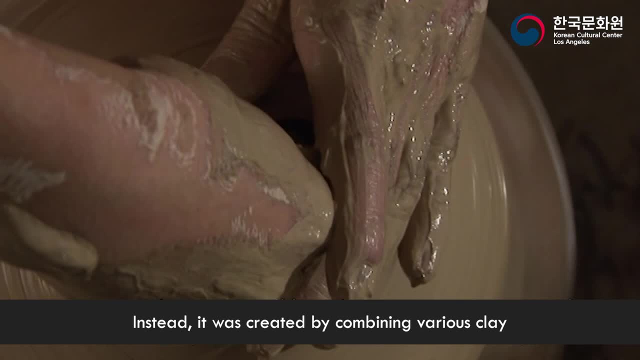 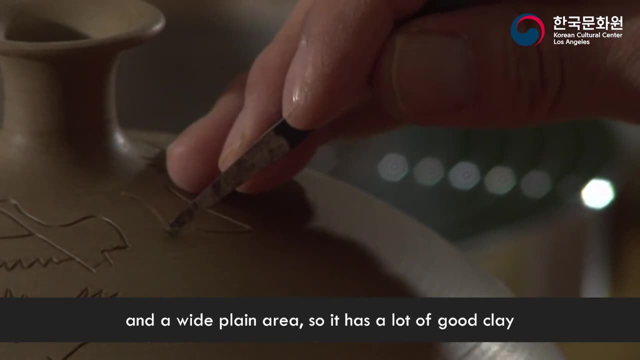 vessels. Instead, it was created by combining various clay in a suitable proportion to make pottery. As a simple example, China has a huge land mass and a wide plain area, so it has a lot of good clay. On the other hand, Korean land does not have large plains. 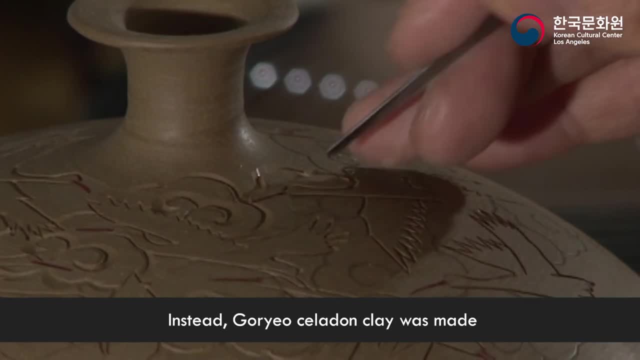 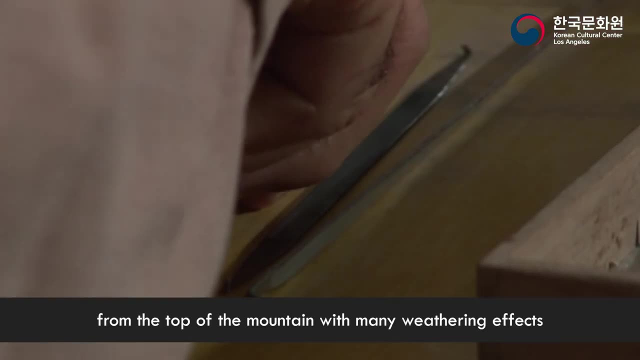 And mountains and valleys are rough. Instead, Corioceladon clay was made by mixing naturally finely ground clay from the top of the mountain with the many weathering effects. This was the wisdom of our ancestors in finding the best raw materials in the harsh and barren. 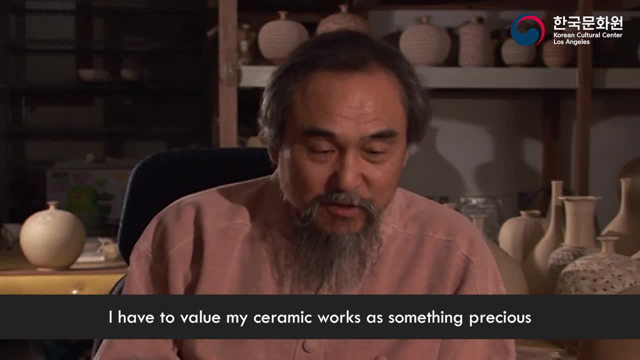 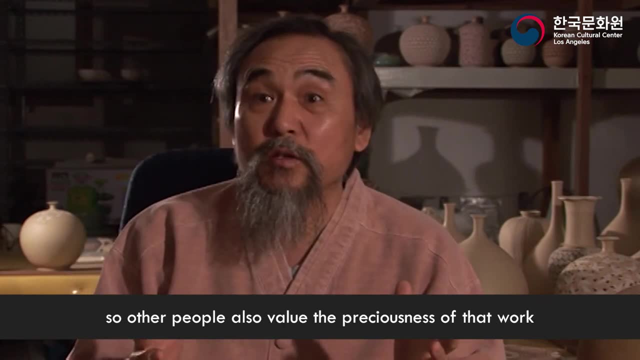 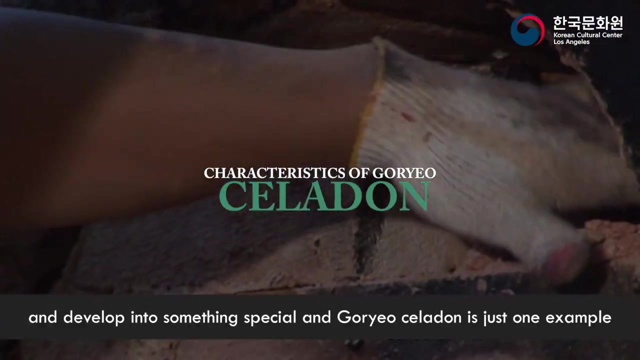 environment. I have to carefully deal with the pottery I made so that other people can see it as precious. That's how I deal with it. That's how I deal with it. That's how I deal with it. Throughout history, Koreans have an ability to embrace small things and develop into something. 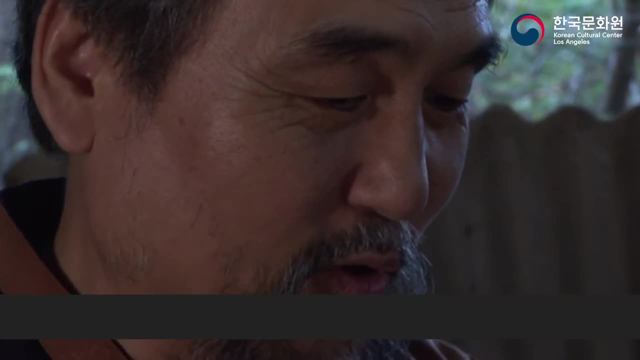 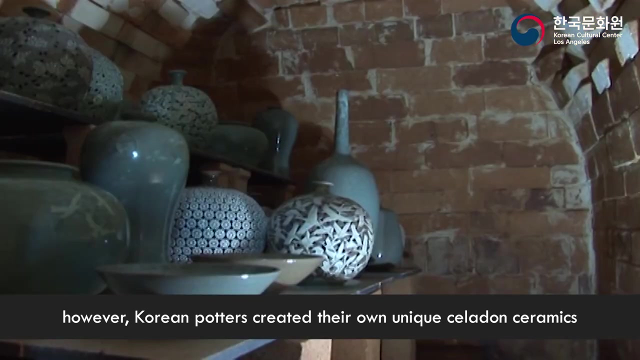 special, and Corioceladon is just one example. Korean potters have been taught techniques by Celadon potters who have been evacuated from China. However, Korean potters created their own unique Celadon ceramics, which some would. 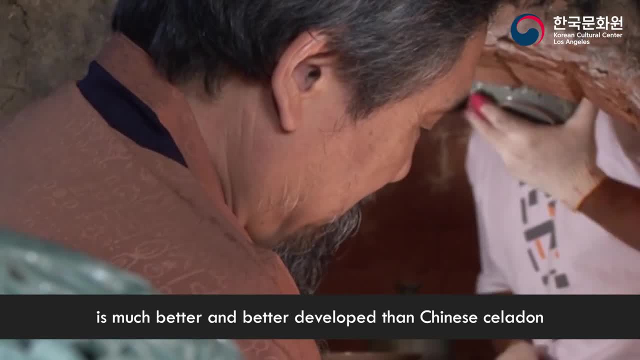 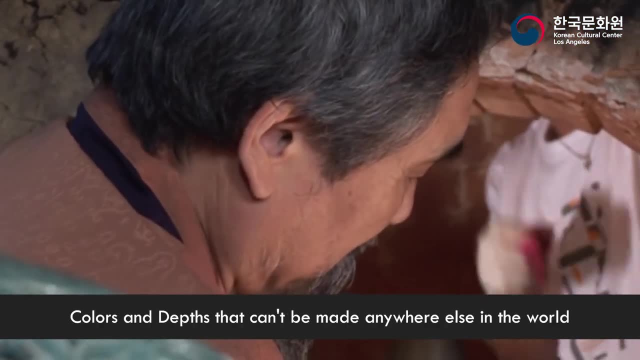 say, is much better and better developed than Chinese Celadon. This is because of their own unique colors and inlaid techniques, colors and depths that can be made anywhere else in the world. This unique color is due to the geographical characteristics and climate of the Korean. 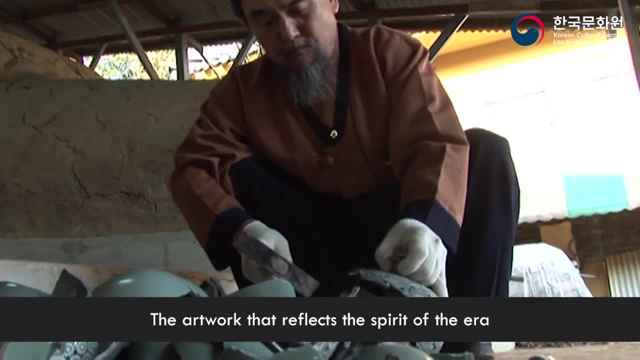 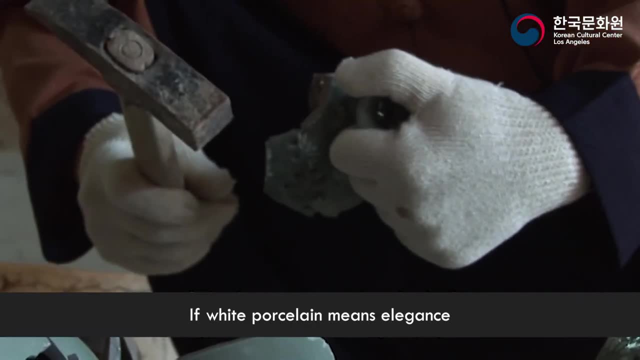 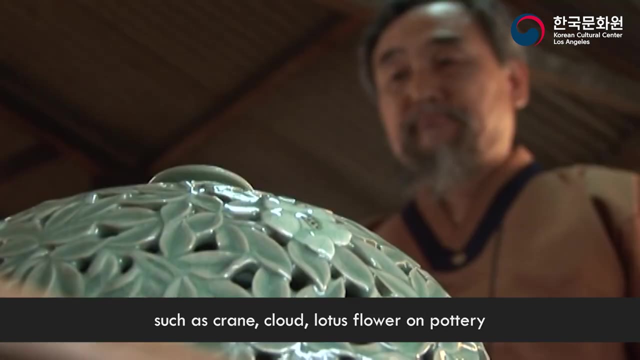 peninsula. The artwork that reflects the spirit of the era was created with designs and patterns based on the oriental philosophy that pursued the spiritual world. If white porcelain means elegance, Celadon is an icon of perseverance and passion. Corioceladon features traditional patterns such as crane cloud, lotus flower on pottery. 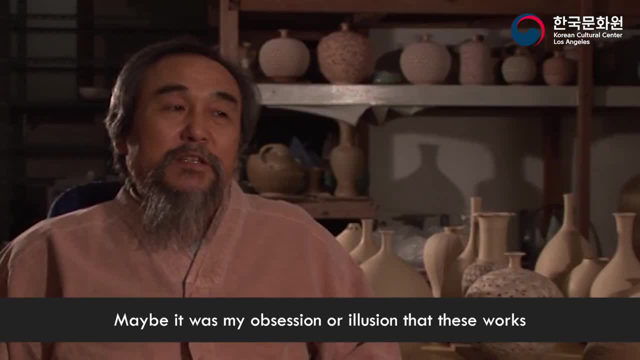 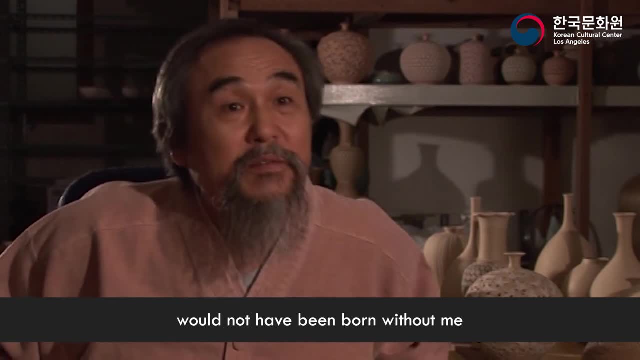 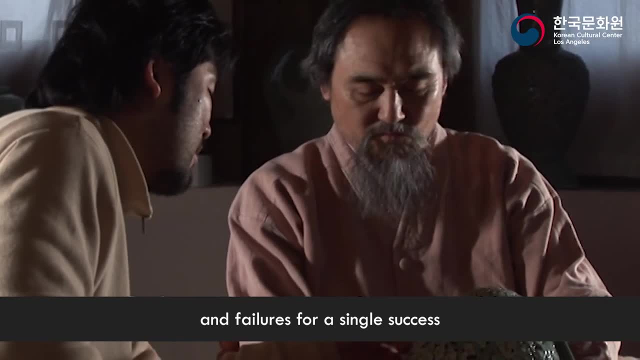 It's a waste. It's a waste. It's a waste. The art of Celadon, its natural beauty, its natural identity, its golden area. How do people experience it? It's a work of art. When one sees the art, it's nearly as weird as the art of the past. 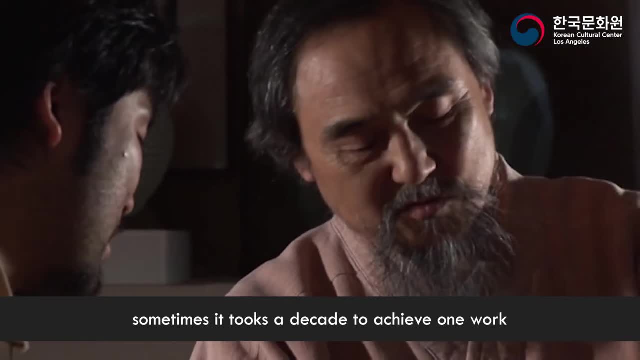 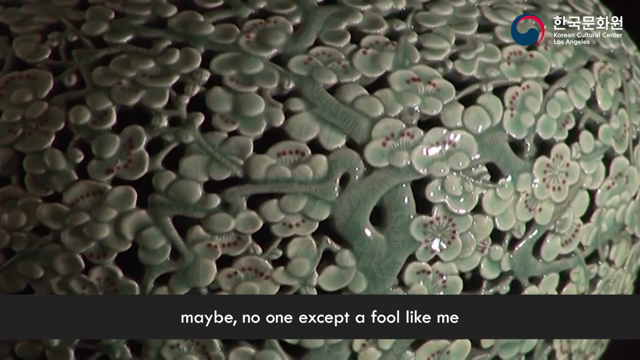 It's a work you can't make. When you think about it, it's an art that you have had for years and also has a certain. There are things that took 10 years to make. Who else would do that? I don't think anyone would do that if they weren't a fool like me. 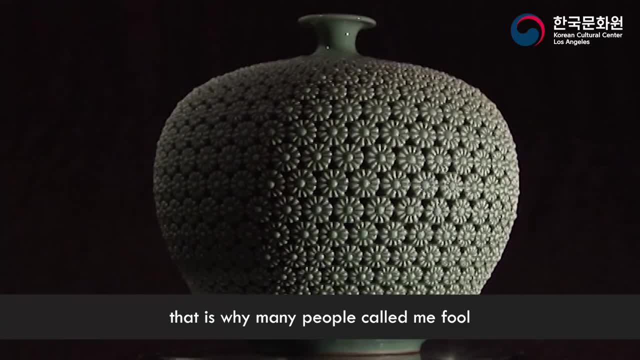 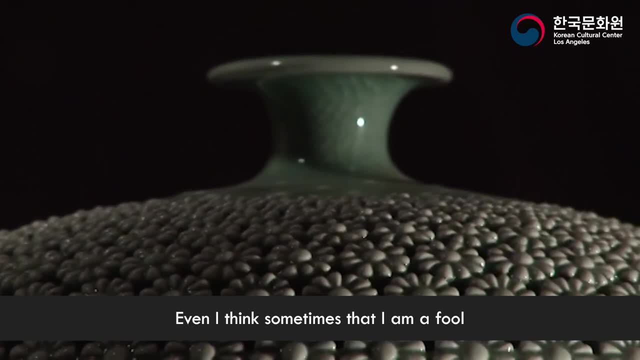 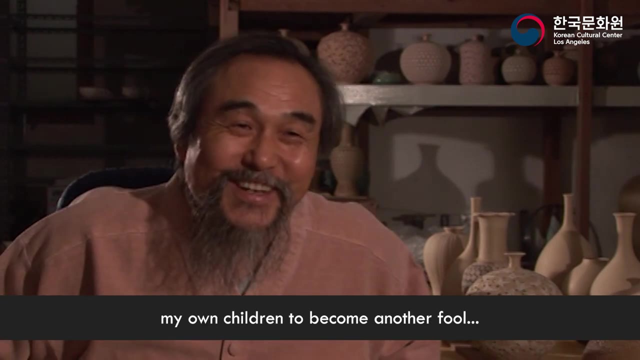 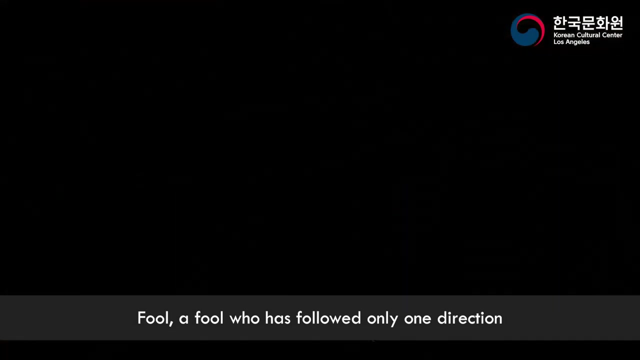 That's why a lot of people say I'm a fool. Sometimes I think I'm a fool, But I don't want to tell my children that I'm a fool. I'm a fool. I'm a fool who only looked at one place in my life.